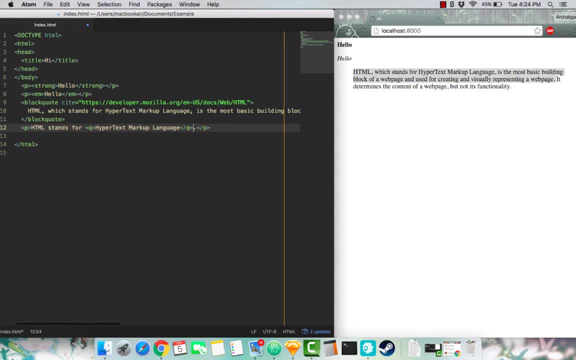 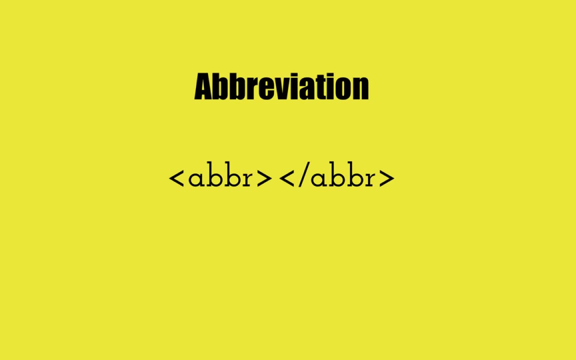 Okay, so Quotes? In a nutshell, it just defines short quotes. HTML stand for, the quote starts there hypertext markup language and the quote ends there. I don't know, we just don't add regular quotes. but what landmarks? Abbreviation: Abbreviation defines an abbreviation. 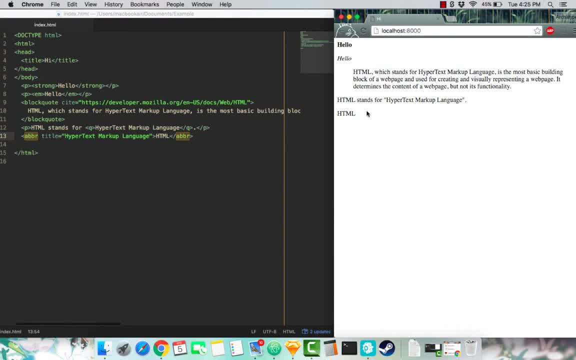 when you hover over it. So I'm going to go here, I'm going to have to click on the browser, hover over it and you see right there, hypertext markup language. the next one is sites. so site, site, in a nutshell, references to any creative work. so, if I 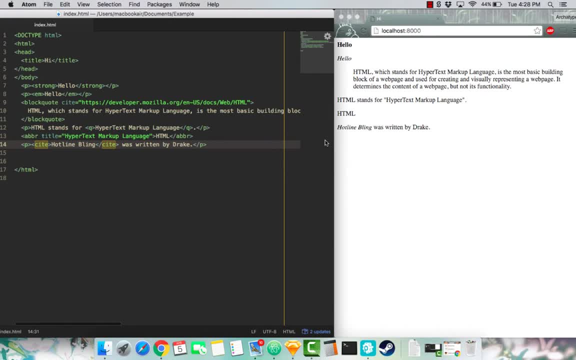 save this, bring it up and see hotline bling and italics, that's it. next one is definition: definition, reprimand. that definition represents a definition term. if I say elf, damn, save that. and then there you see programming in italics. I actually I should turn this comma into a: that's there we go. that looks better. 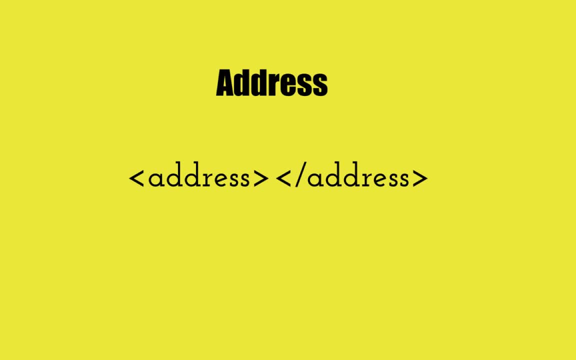 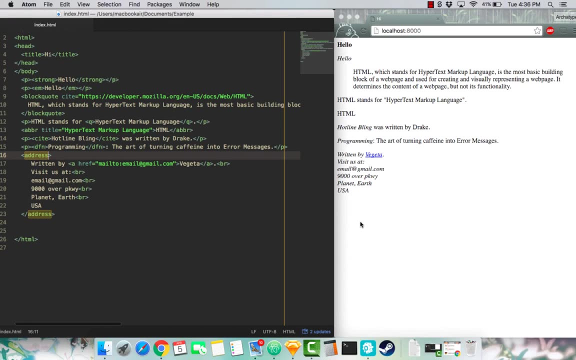 next one. so address defines the contact info for the author of a document or article. so I have one right here. if I save it. everything's written in italics right here. so deletes and inserts. delete and insert. okay, let's start off with inserts. insert defines a text that's been on inserted into a document. hence 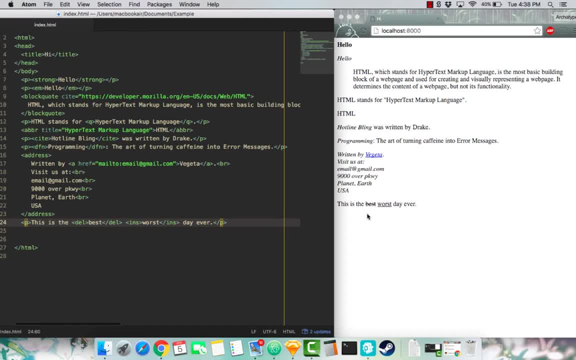 the underline in deletes defines a text that has been deleted from a document, hence the crossover or a strikethrough. so the last tab will be the s tag s is um short for strikethrough. at least I hope so. and you may think that this is similar to the arm deletes. well, it's similar, but the s?